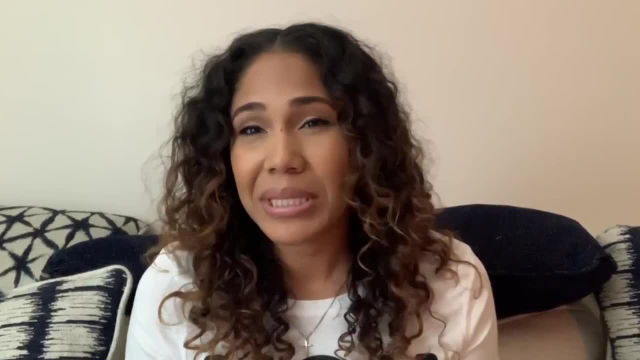 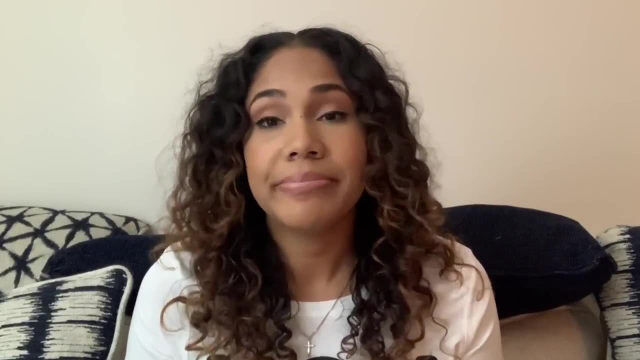 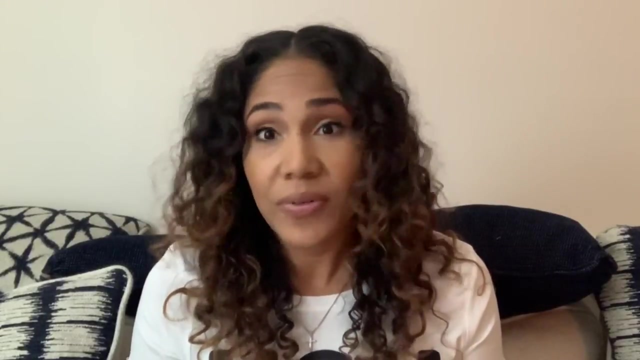 to be autistic. I don't really like the way that they did that. I do feel like Ashton might be somewhere on the spectrum, Um, but you know that's what they said, So we're going to he gets checked again, I think, in like two months to see, and hopefully by then when they see 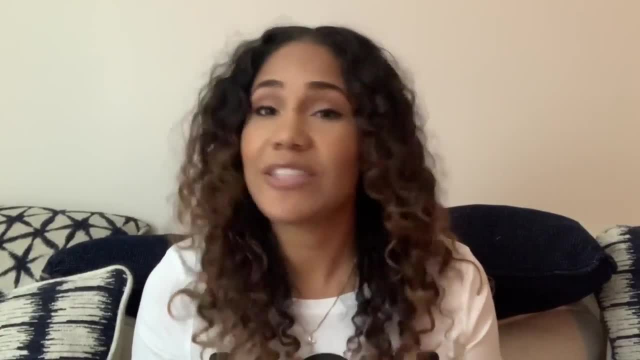 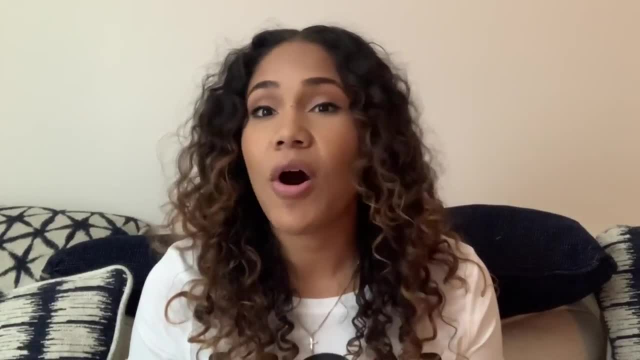 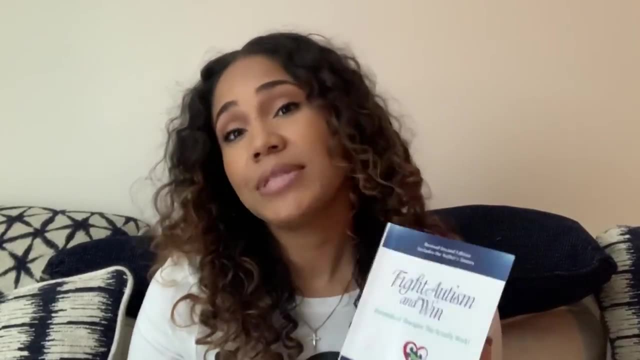 still keep on moving forward and he will still be on this great path of progress, And I just know that God has his back. So but the reason why I use this book- it was actually recommended to me- It's called Fight, Autism and Win And it's basically biomedical therapy for your kids. 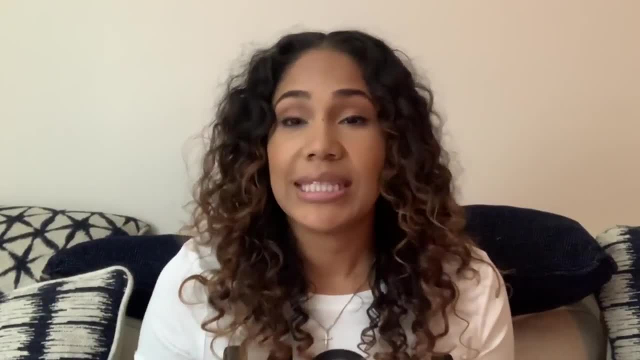 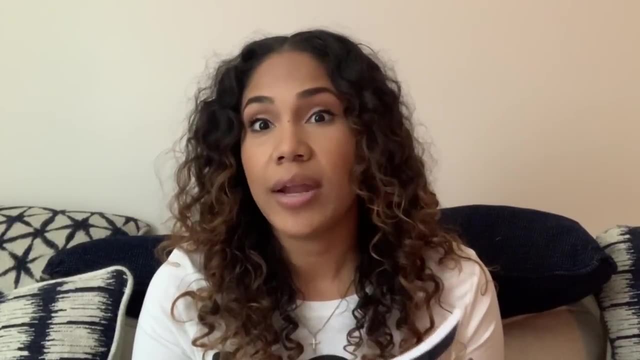 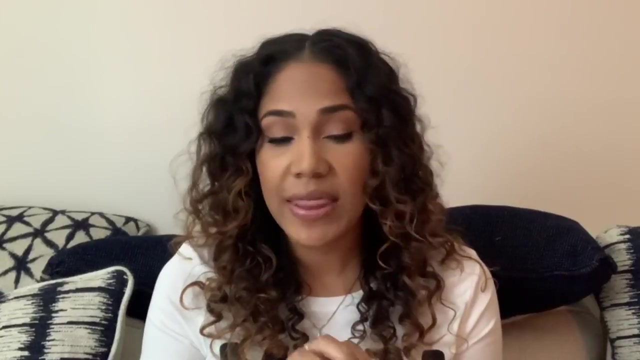 which is like incorporating all of these vitamins and doing all of these things. Now, I really do like this book because it really does- um, it really does inform you a lot about different vitamins and supplements that can really benefit your child. Then it goes into something called chelation, And that is basically when you are 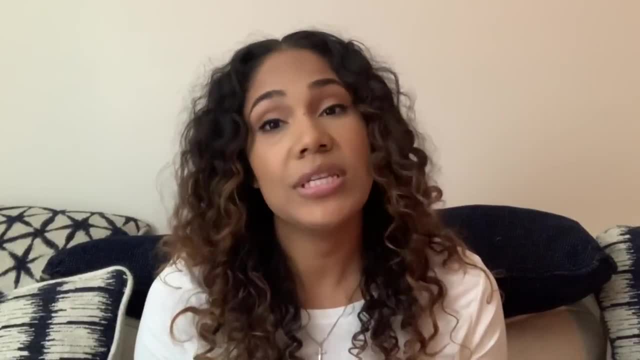 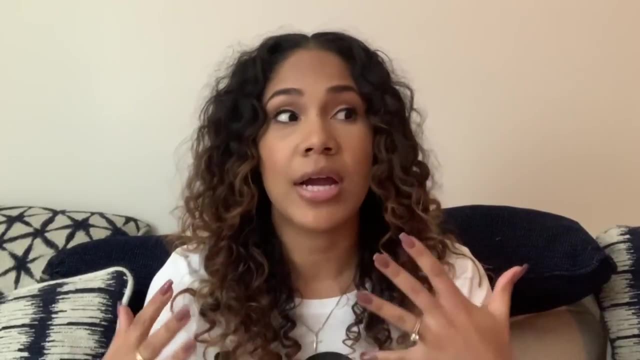 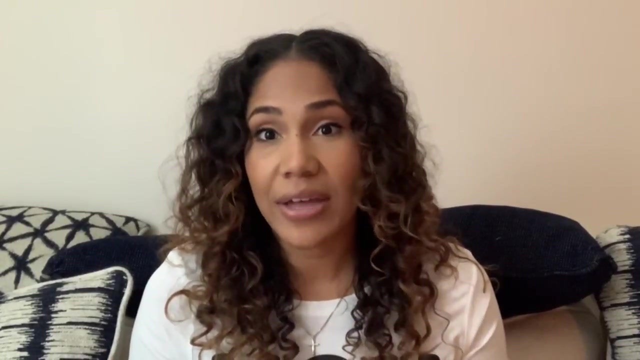 slowly drawing metals out of your child's system. The reason why this is important is because a lot of times, children have a lot of metals in their system that are that people assume it means that they're autistic And it's because these metals can cause the child. 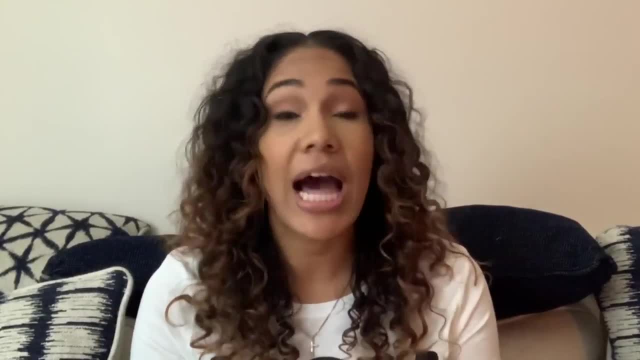 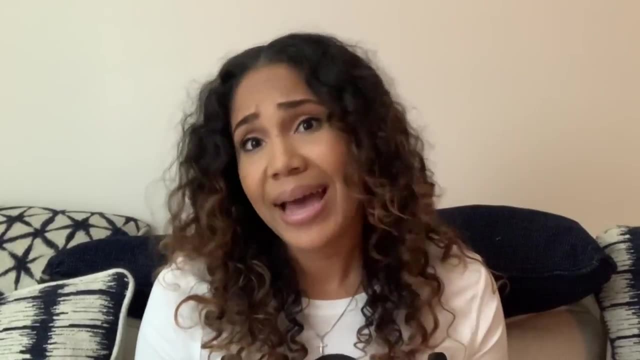 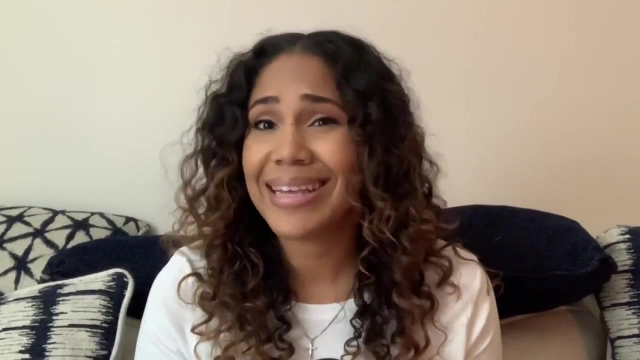 to display autistic like qualities. a lot of them. Um, and so the first thing the book tells you to do is to get your child tested. I got Ashton tested, We got his hair tested and we did a saliva test. Basically, you pay for the test. The tests are like. they ended up being around $400,. 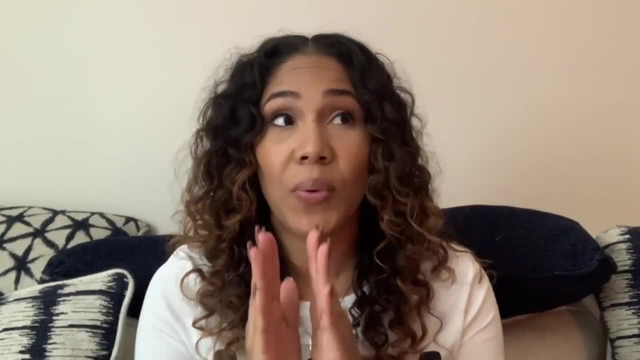 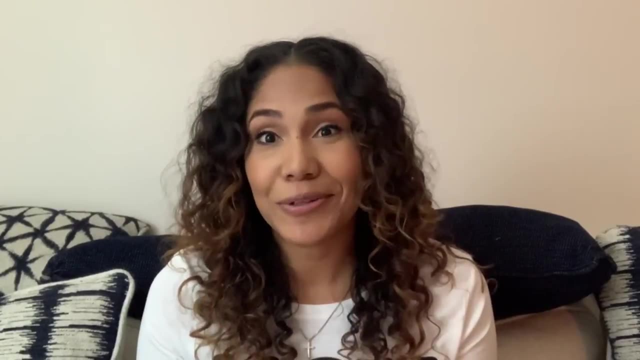 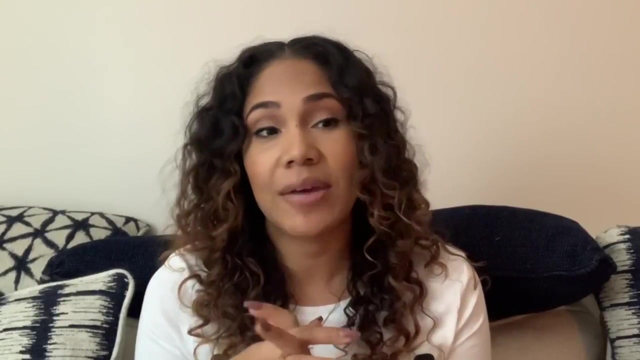 but it's worth it. Um, so I believe the hair test was like $250 and the swab test was $150.. When we caught our results back for Ashton, he was mercury toxic and he had very high aluminum levels. That could be anywhere from the water that you're giving them. That can be from their mattress. 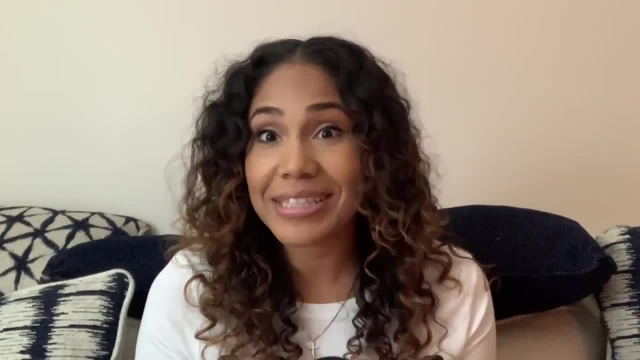 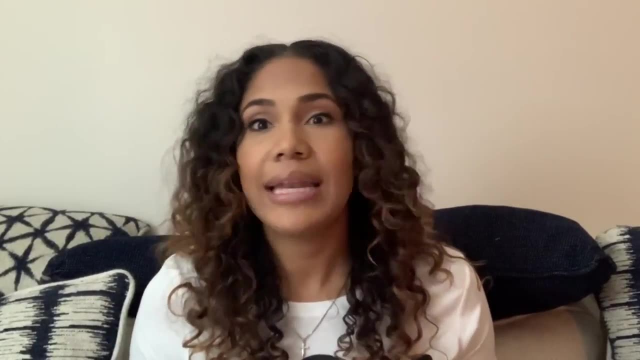 the type of mattress they're sleeping on. That can be from the type of pajamas that they're wearing. There is different things that you would never think that can truly affect your child. So I had to get hip to all of this stuff, to what this metal, these metals in the system meant. 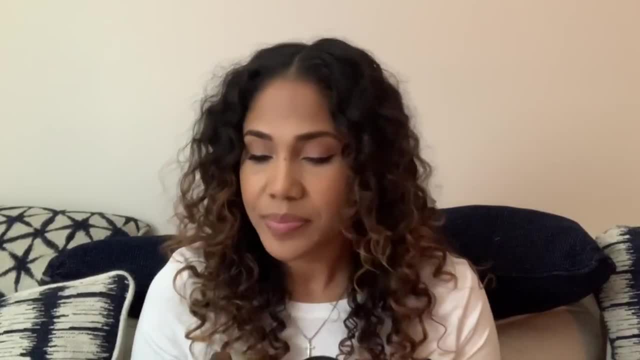 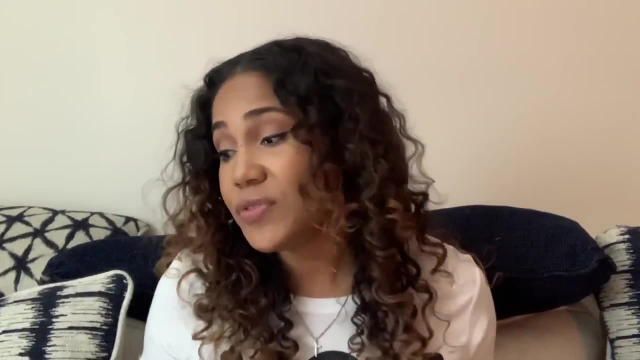 and how I could get them out. So someone else recommended something for me that I'm going to tell you guys in a little bit, And that's that's the route that I went. So I kind of use some of the vitamins and supplements. 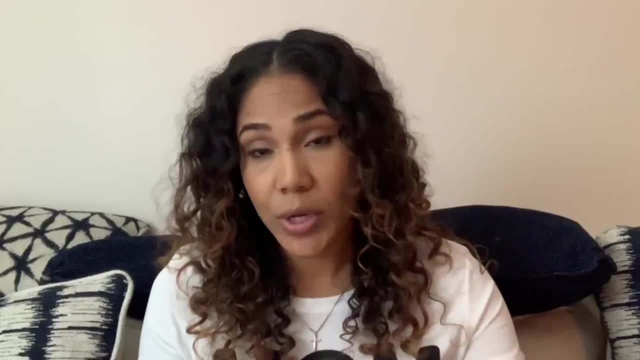 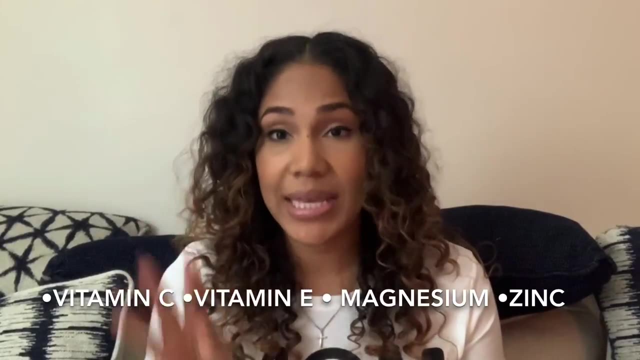 that this book says, And then I I kind of went and did my own thing as well. So the first thing it says is that you need to do a core four. So the core four is vitamin C, vitamin E, magnesium and zinc. Now they in the book. it tells you to give them so much. 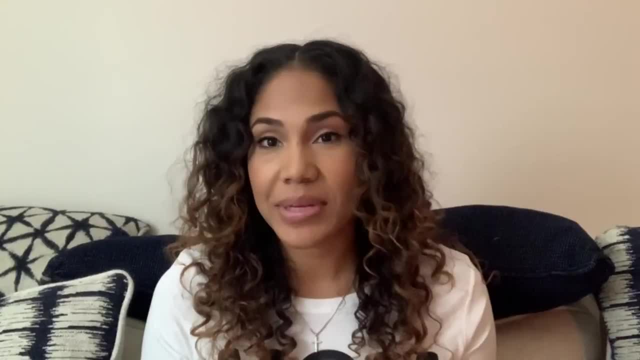 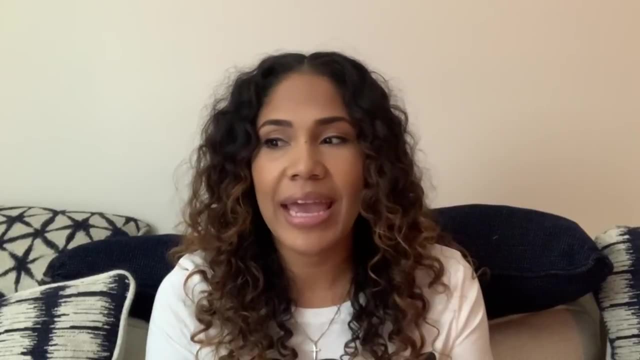 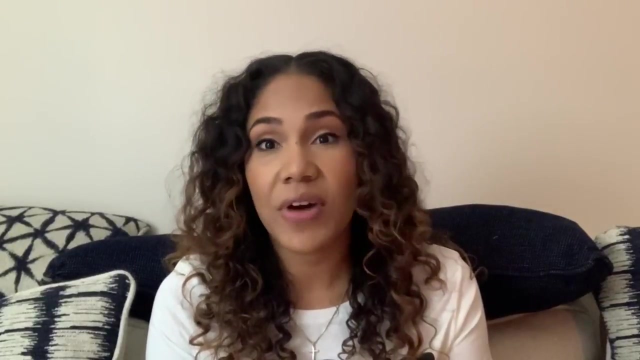 Um, it's alarming How many vitamins, how much of each vitamin, you're supposed to give them a day. And at first I did do it, Um, and I just didn't feel comfortable with it. I did it for maybe two and a half weeks, And my um stepfather- he is a doctor. 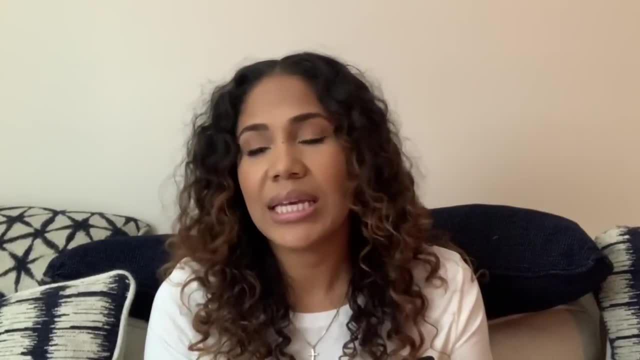 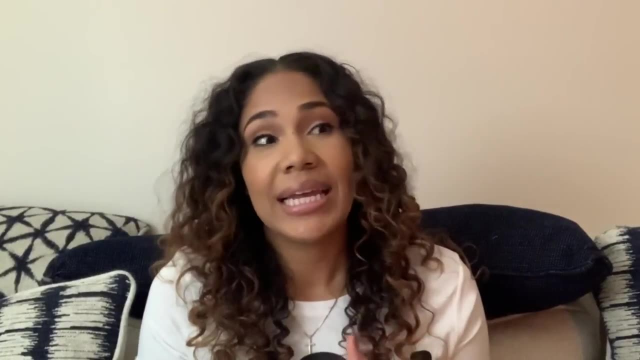 And then I went and talked to him about it And he was just like you're: once your body has an excessive amount of vitamins, it just gets rid of it. So you're just putting this inside of his body and for no reason. 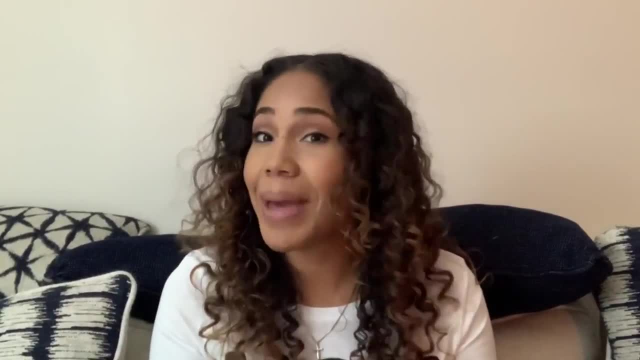 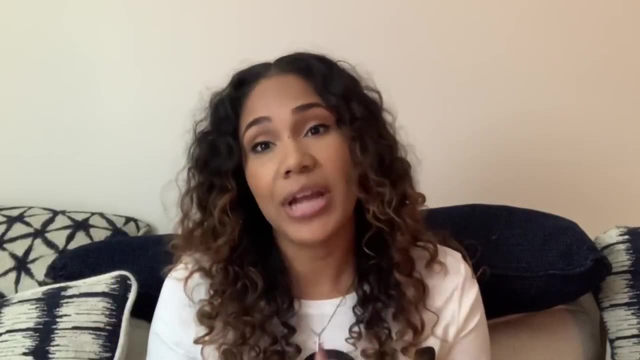 and you don't know how it can harm him. So I took it back a lot. I ignored the book on how much I use what it said to use, but I ignored how much, And, um, you know, so I've kind of changed it. 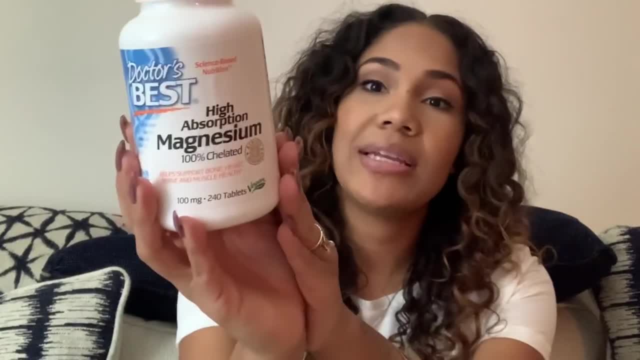 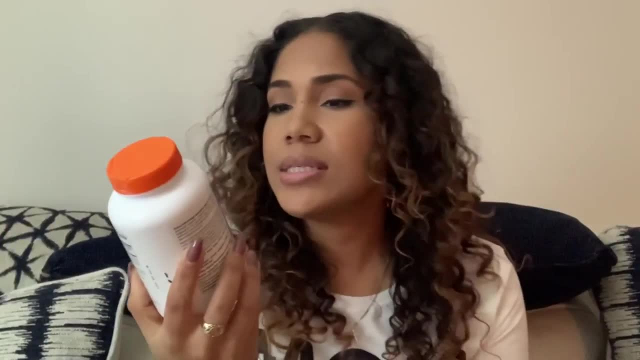 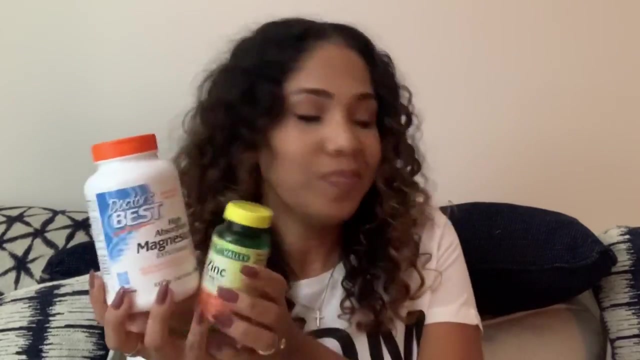 So what I did was I bought these. this is the magnesium that I use, and you want to use the, the chelated magnesium, And this is like the regular adult magnesium, So I use this one zinc, vitamin C, and then the vitamin E is in gel form. 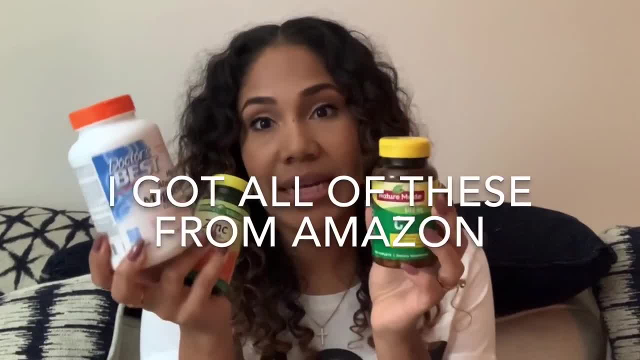 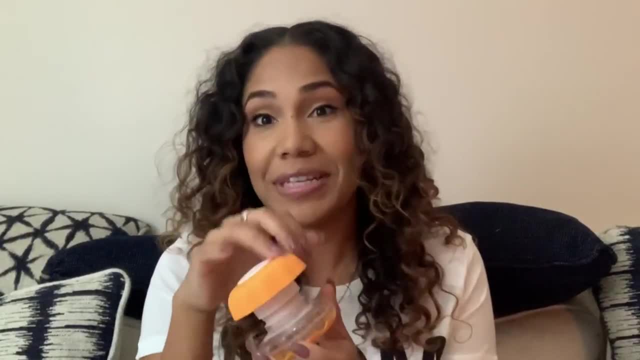 And that's downstairs And I don't feel like going to go get it. So I know you're wondering how I got it to get a toddler to use these. So I literally have to crush and grind all of his vitamins every week on Sunday. 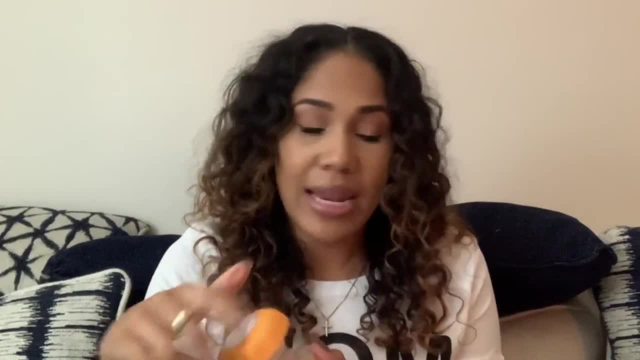 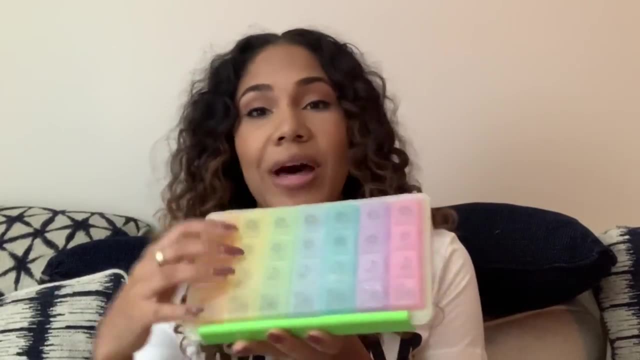 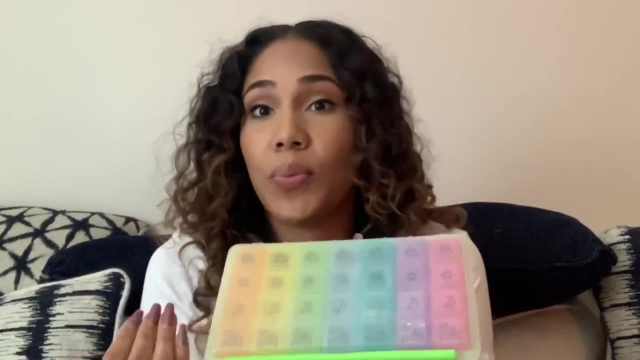 night I crush and grind all of his vitamins in here and I spread them out in this pill box. So this pill box has all of the it has every single day and then it has like the four different days. I got this from Amazon. It just happened to work with what we're doing. 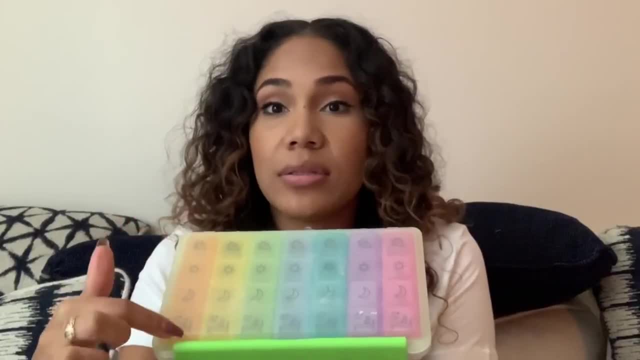 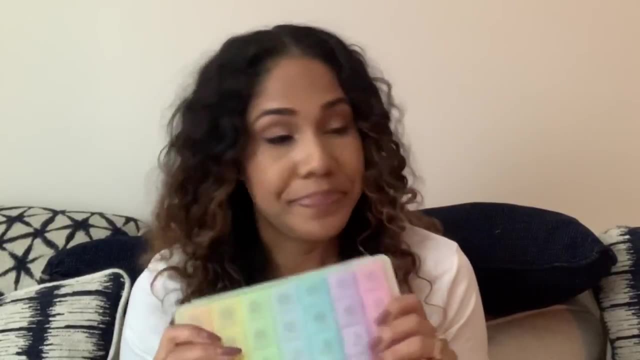 So it has the um four different doses for each day, So that way I know if I miss a dose, if I forgot you know anything like that. So that is his core form And that is what he does every single day, four times a day. 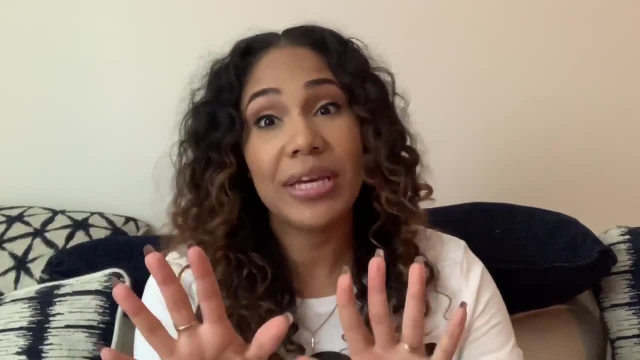 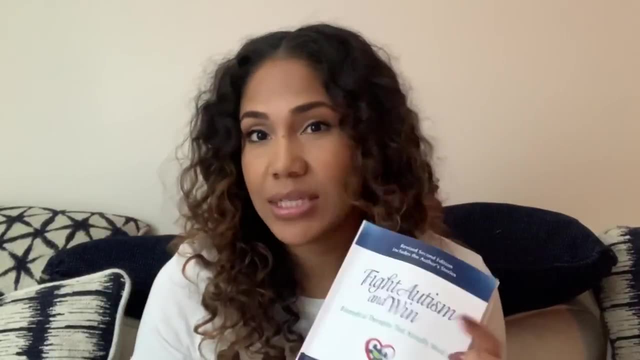 The reason why I'm not telling you how much of each is because that's totally up to you And you kind of have to um play around. And I really do think this book fight autism and when it is really important because the book really outlines what each vitamin does or what he supplement. 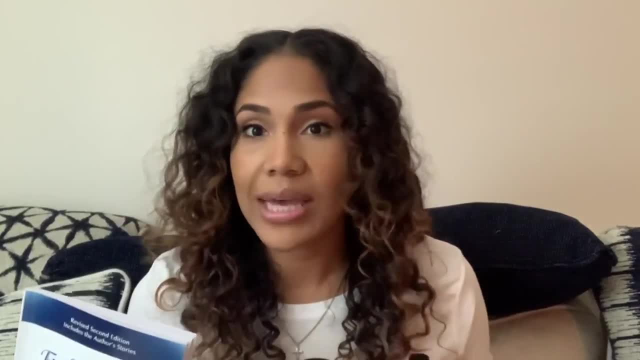 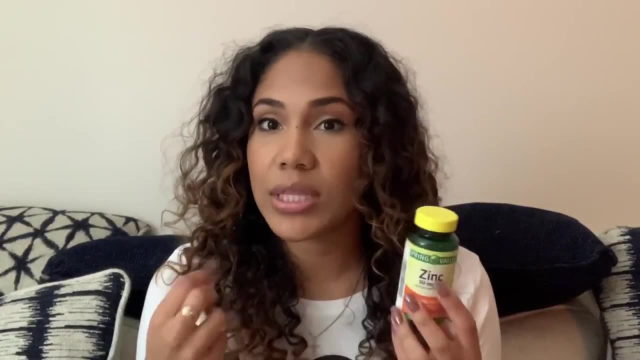 does Um. for instance, Ashley used to grind his teeth all the time, not when he was sleeping, but just like when he's just like sitting there, and he was just grinding his teeth, especially in the car. think it's something that really helps with his. 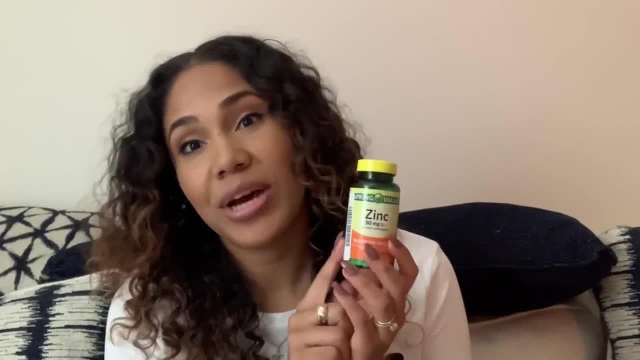 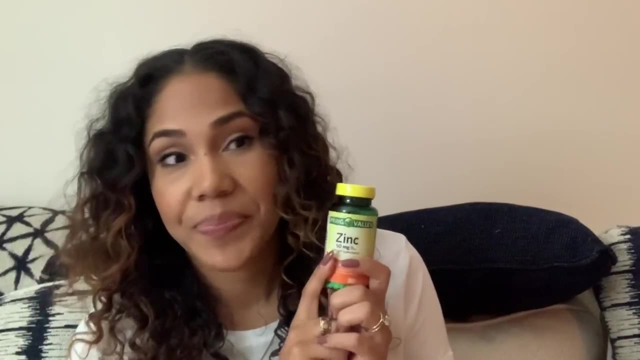 him grinding his teeth. So but you don't want to give too much. So, for instance, the book told me that Ashton should take 50% of his vitamin and not twenty percent of his vitamin. milligrams of zinc a day, my stepfather said he doesn't even recommend more than. 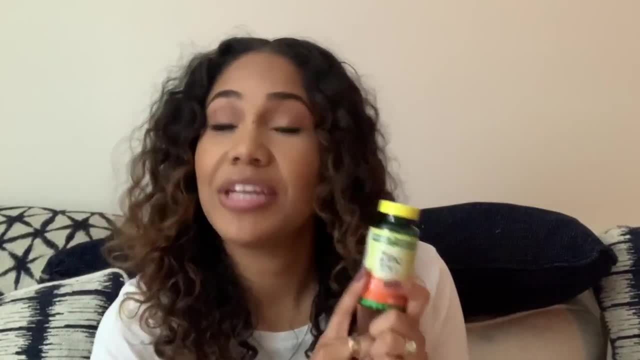 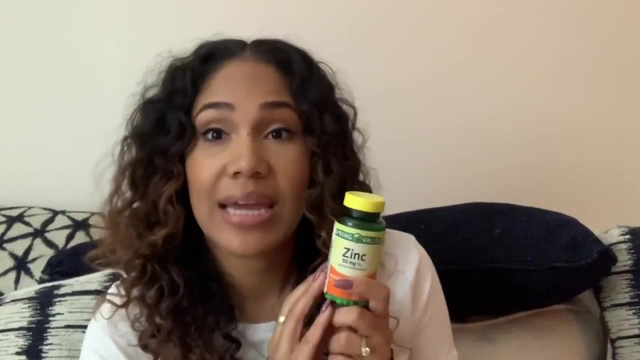 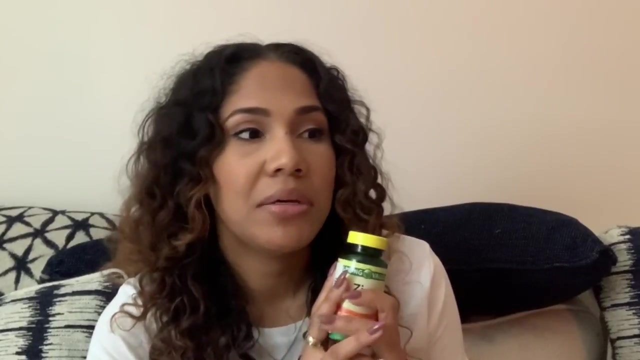 15 milligrams for an adult, a regular-sized adult. so for Ashton, I gave him about ten, five to ten milligrams a day of zinc and it has really helped. he does not grind his teeth- teeth as often. maybe, maybe every three days he grinds his teeth and it's not for as long. before in the car he would just grind. 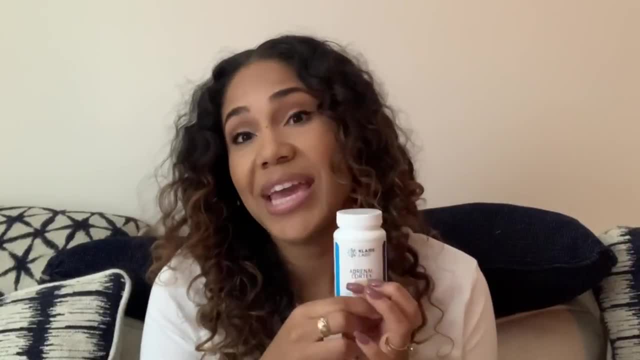 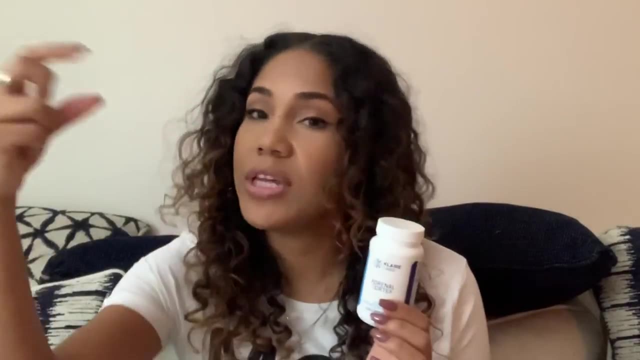 his teeth the whole time and it was so annoying, but now he does. so. the book has a page that has all of these additional supplements other than the core fourth. that could really help your child. but it tells you like different things, like for this, for that. you know what? one of the things that I really love is this: 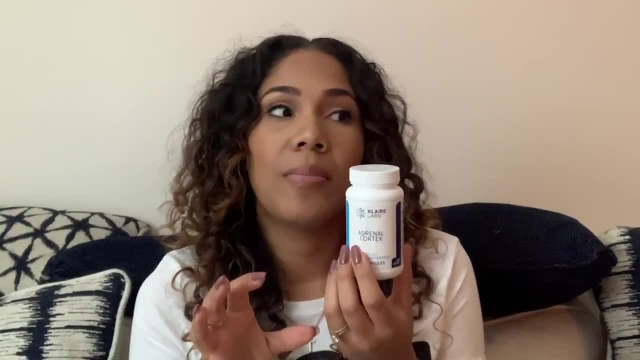 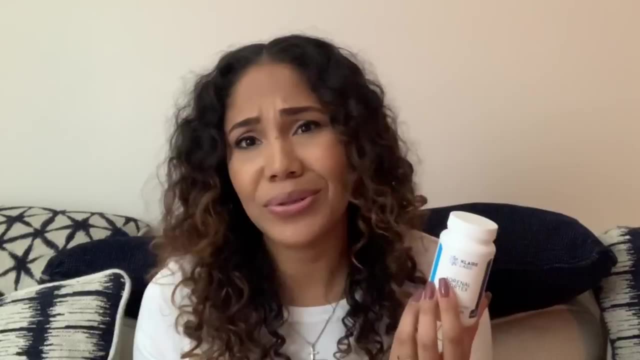 adrenal cortex and this really helps a child who's super, super hyper, Ashton, is gluten intolerant, so he has any kind of gluten, which there's always gluten in my house because I buy. I buy all of his food foods gluten-free, but his brothers have stuff so he doesn't have any gluten in his food. so he doesn't have any. 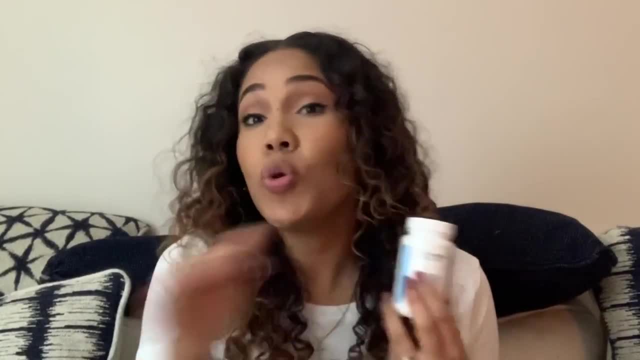 gluten in his food, so he doesn't have any gluten in his food, so he doesn't have. sometimes he'll sneak stuff out of their bags and I can tell because he's super hyper, he's a little bit of gluten and he's off the walls bumping into things. 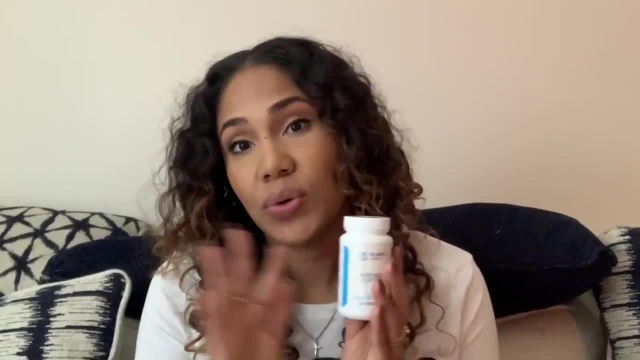 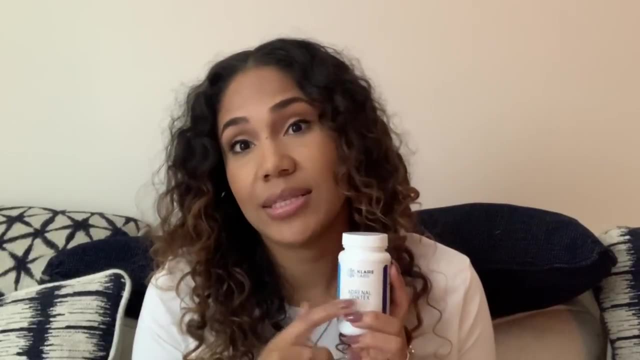 breaking stuff running back and forth. so this really helps to kind of calm him and keep him, you know, just balanced throughout the day, and it really helps with me doing his speech exercises because it helps him to kind of sit and listen to what I'm saying. so this is adrenal cortex. this I had to order. 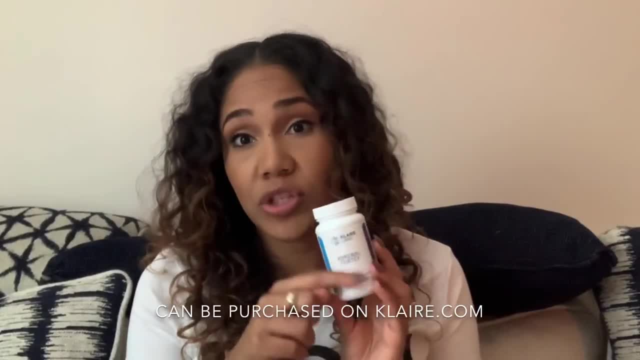 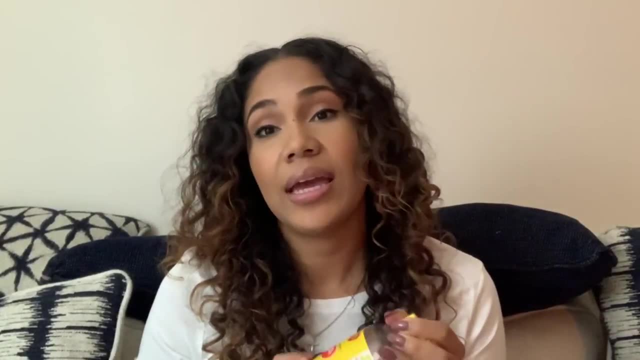 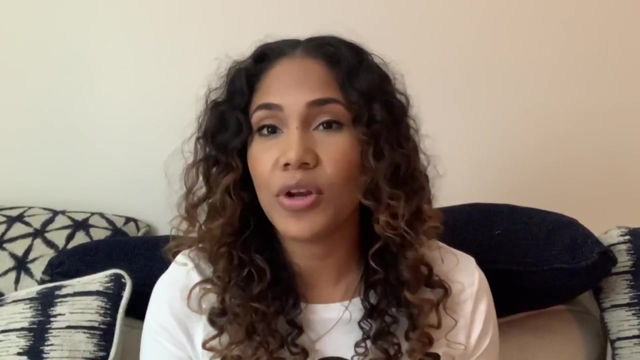 online from Claire laughs. like especially from Claire laughs, this is one that was very highly recommend. so, because Ashton is on a gluten free, dairy free diet, I want to make sure that you have the things that he is missing with you know, being on dairy-free diet, I did learn or see that after we took dairy away even. 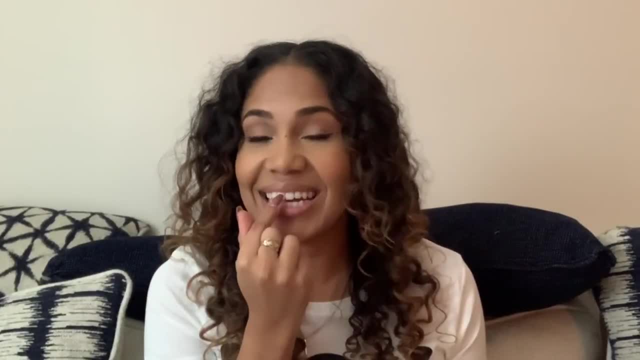 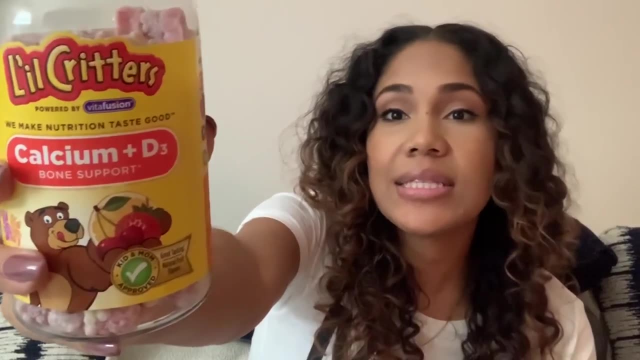 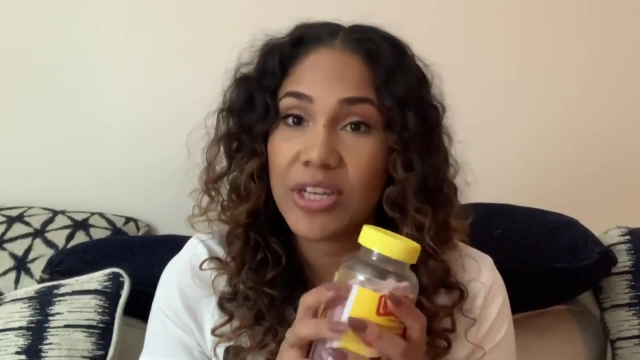 though it made a big change in his teeth. you can kind of see that he's lacking, you know, the calcium that he needs from dairy. so I started incorporating these little critters- calcium and d3 vitamins, which works so well with ashton, because you can start to see his teeth are. 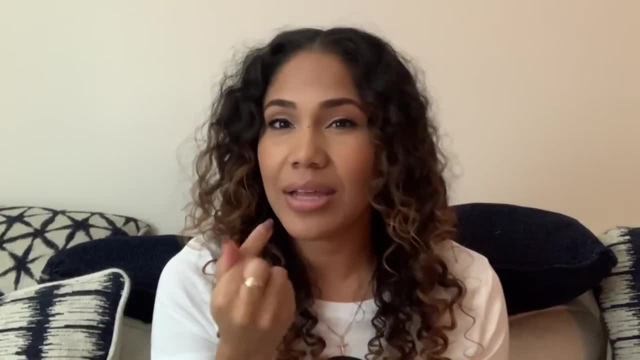 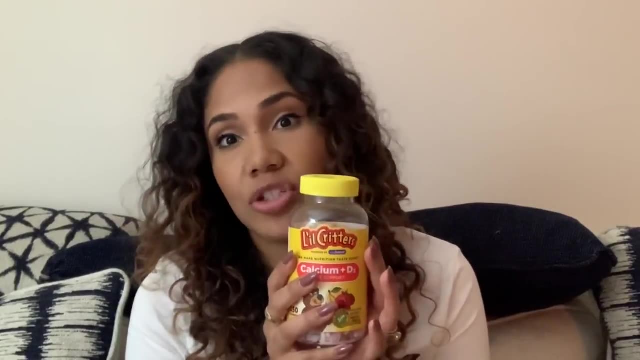 getting white again. not that they were really messed up, but you know, you can tell like if the person doesn't drink enough milk or have enough calcium. that was what was happening, and now all we can totally see a change already, and he's been on this for maybe like um, maybe three weeks. 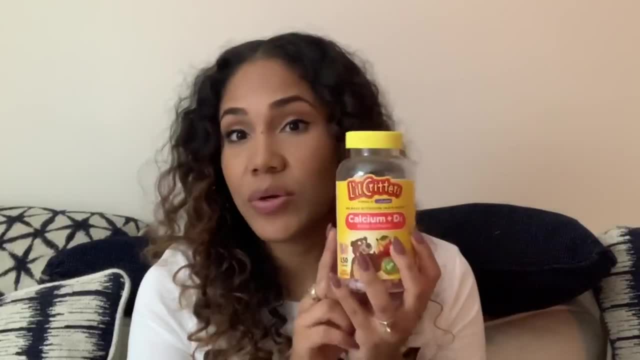 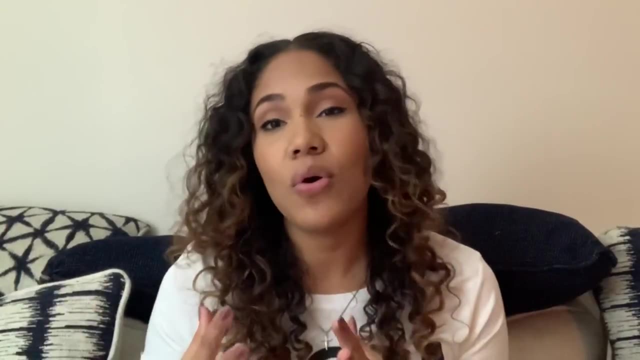 almost four weeks. so, um yeah, these are just little gummies. he likes these. he has two every single morning. okay, so now to the chelation to get the metals out, because all the core four does is prepare your body and make sure that your body is strong for when you're trying to remove these. 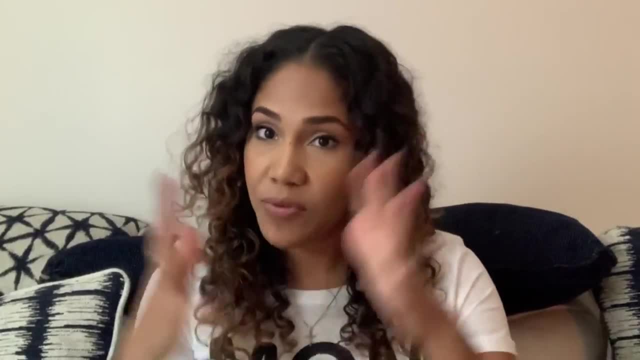 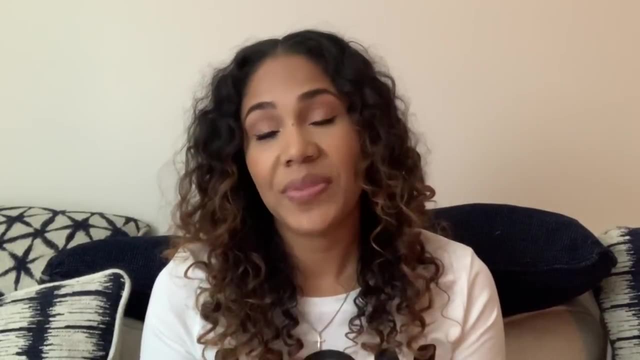 metals, because removing these metals that are in their system from my research i could totally be wrong, but from what i've gathered, the metals attach themselves. they're in the bloodstream and they attach themselves to different organs in your body. a lot of them are in the brain, which 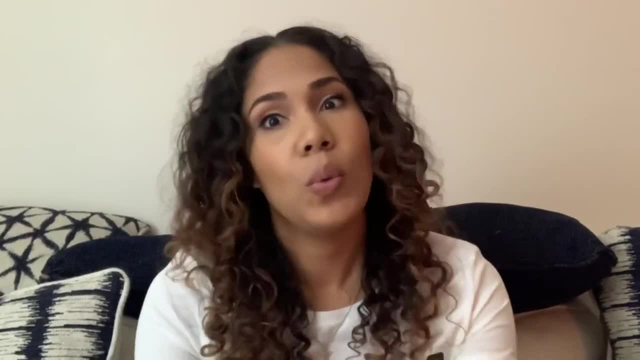 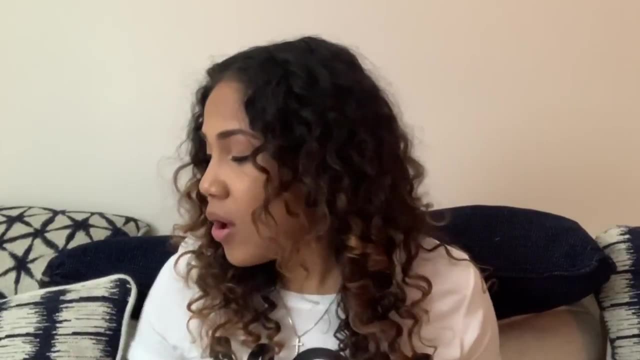 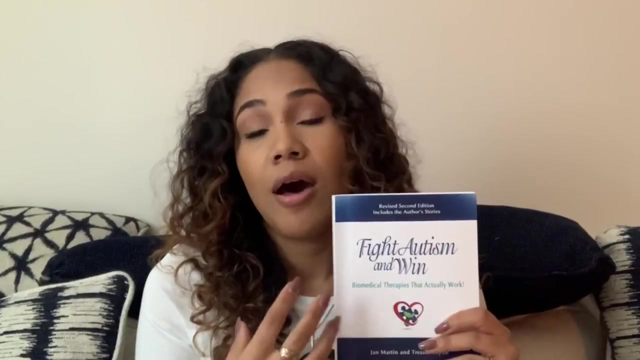 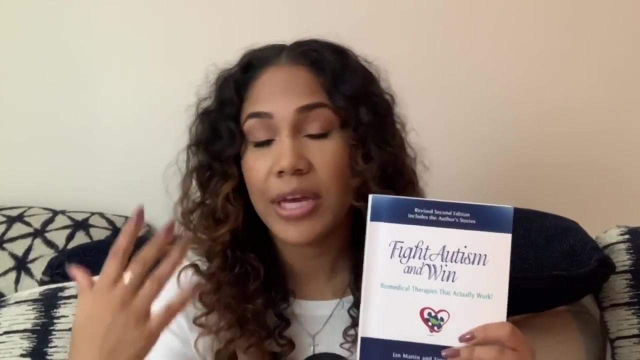 blocks the way that a child's develops and grows, which is very important. so once you start to remove them, you'll start to see your child start to catch up. now the fight autism and win book has a very- they say it's a gentle way to do it. um, it's called chelation, like i said, and basically for three days in a row they encourage. 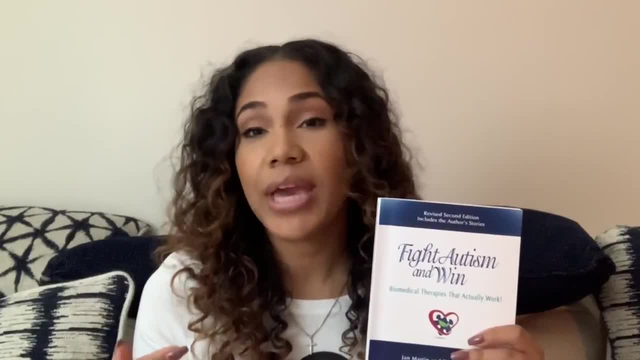 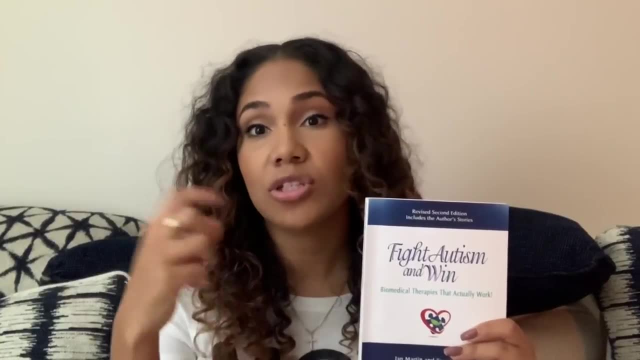 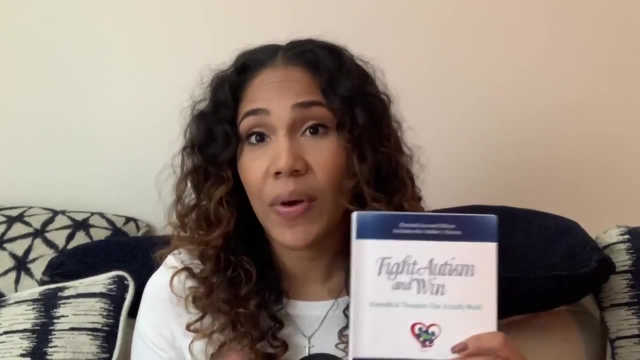 that you do it every weekend, um, every three hours, you give your child this little dropper of this supplement that starts to kind of pull out the um, the metals in their system. but that means even throughout the night. you have to do it too, and so it was something that i was gearing for him. 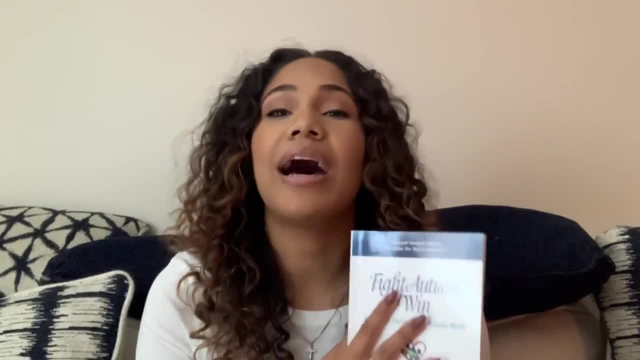 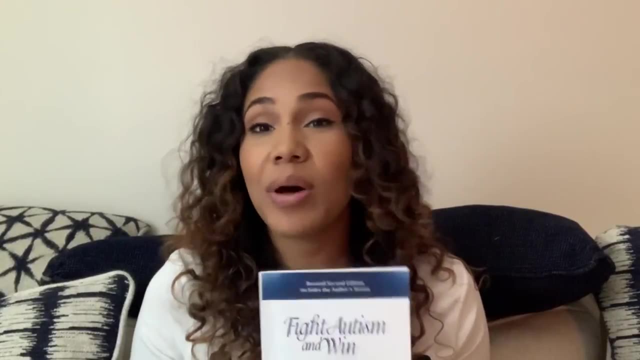 to do. i started doing all of the prep once i got it, but i just could not wrap my head around doing this three for every three hours, like i just could not. i'm a mom of three. i am a full full-time working mom, um, my husband and. 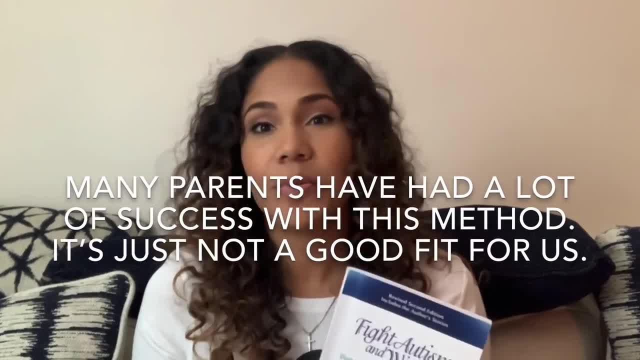 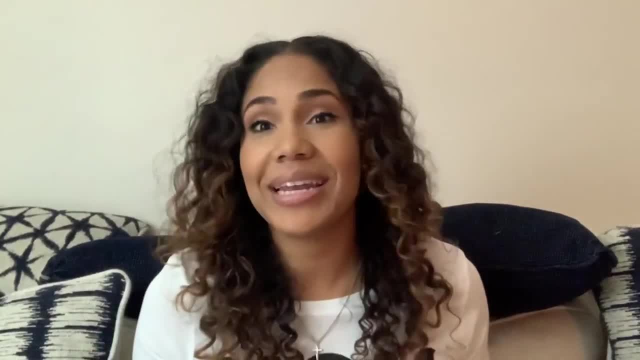 two businesses. i don't know how we would really be able to do it and it wouldn't affect our work life. it wouldn't affect our other kids. i'm just not about that life. so someone recommended, and i for the life of me i cannot find who recommended it to me, but i'm forever grateful. 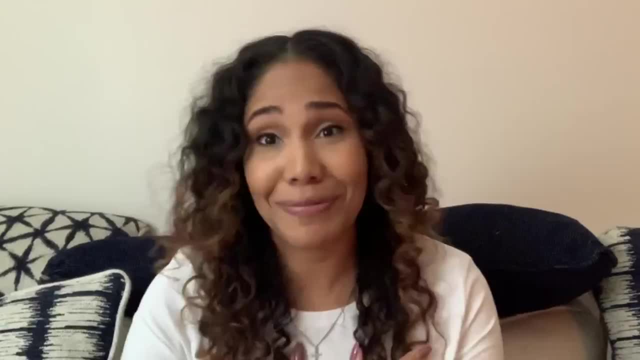 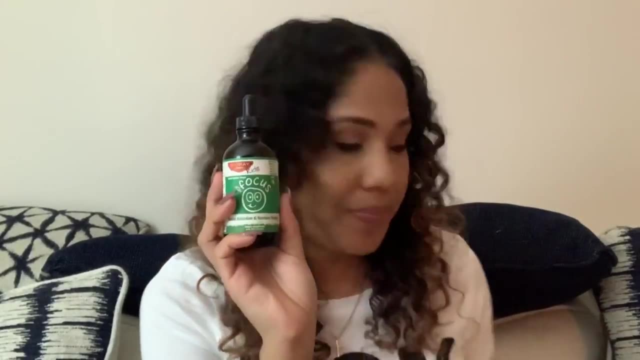 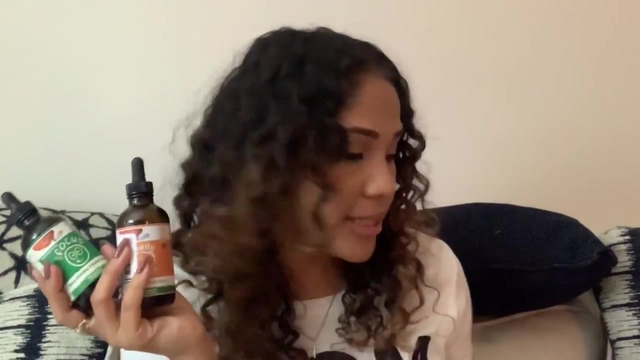 to you and if it was you, please let me know, because you have changed my life um a brand called biore. so this is bio biore, and there are these little drops that you can put in your kids um like drinks in their juice. that's how i put. that's how i give ashton all of his vitamins. i put. 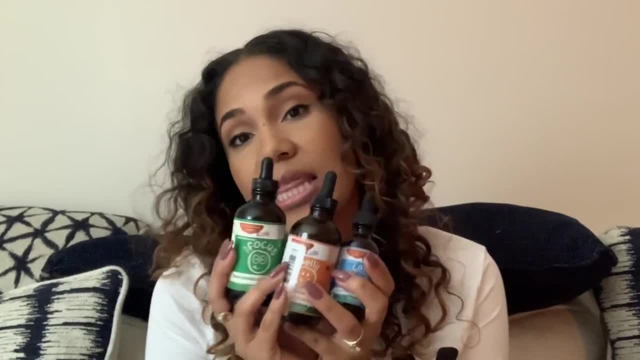 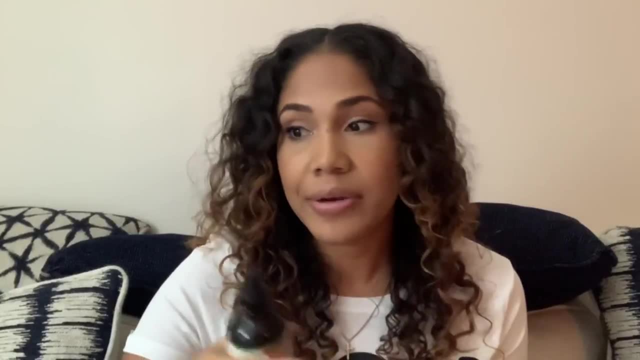 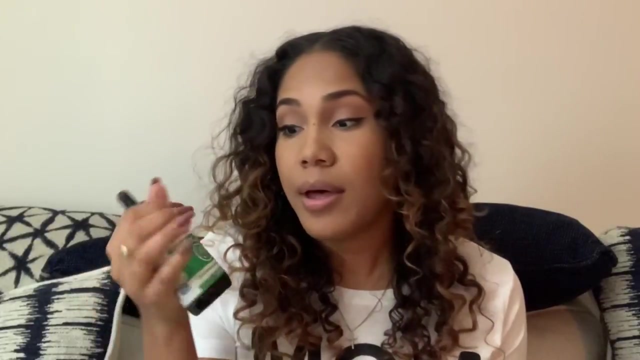 it in his juice. so these drops he gets in the morning and at night. but you have to incorporate them, like you give him one for two weeks and then you can incorporate another. biore has a whole collection of, um, different drops for different needs. but the whole point of biore is to safe. 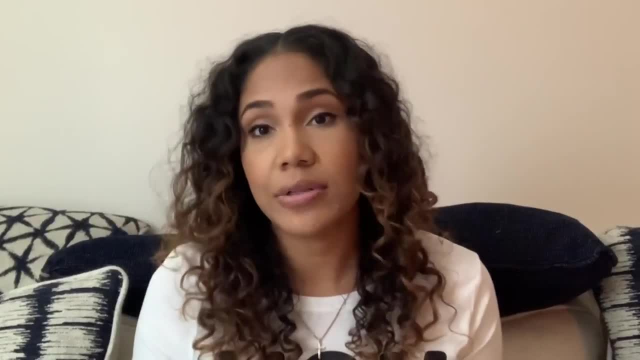 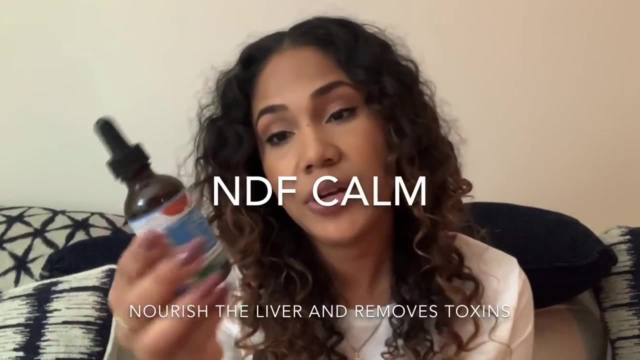 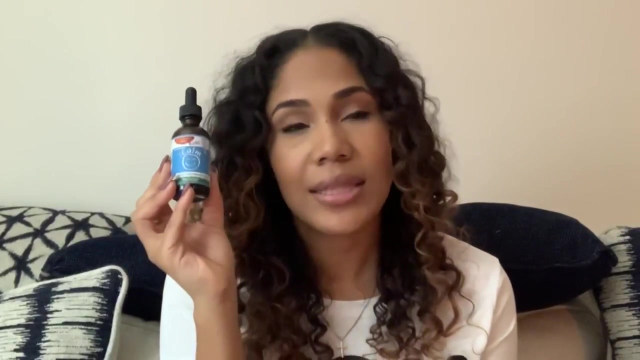 safely remove metals from a child's system. so what we started- with which with ashton- is a calm, so this one is to nourish the liver, and it helps to remove the toxins, too. the reason why it's important to have something that protects your child's liver is because the metals coming out are going to come. 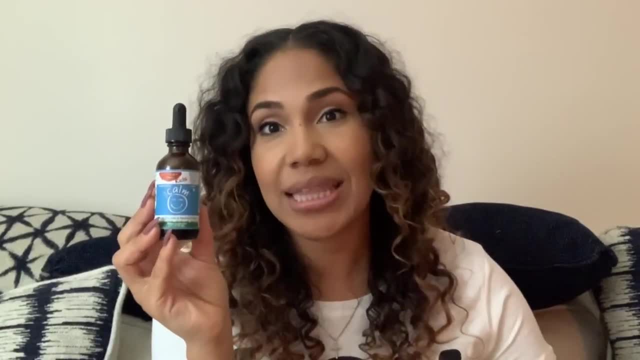 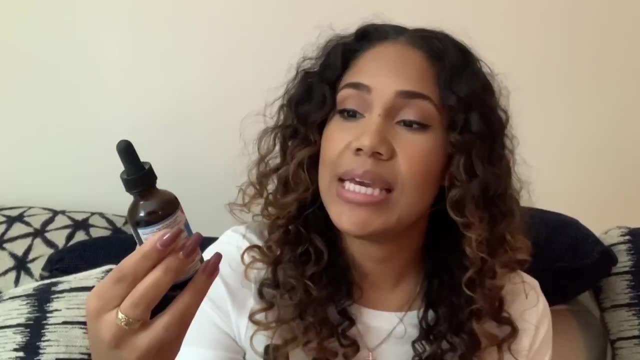 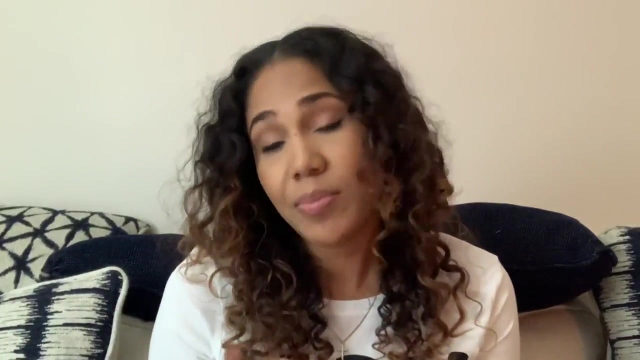 straight through the liver and you don't want them to just start collecting in the litter liver. so you want to make sure that the liver is well protected. so this is the first one that we started with and this is the. it's called mdf calm. so we use this one for two weeks before we then introduce the belly balance. the belly balance is: 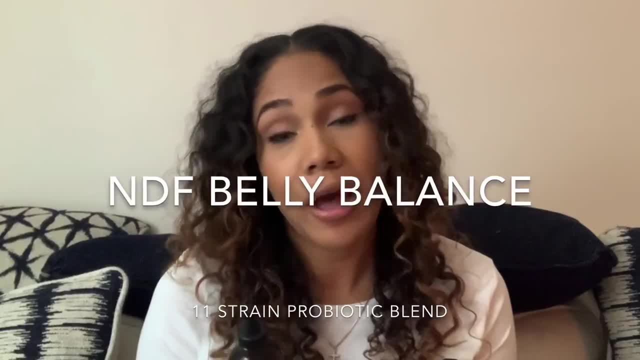 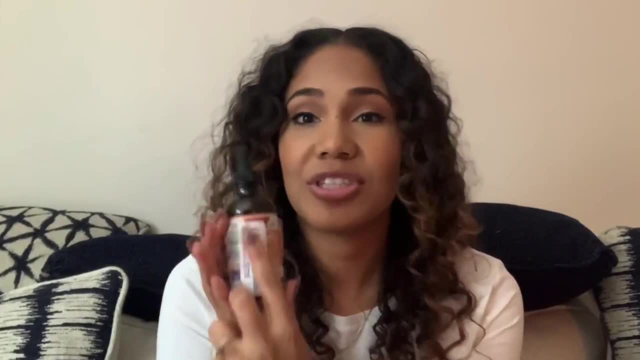 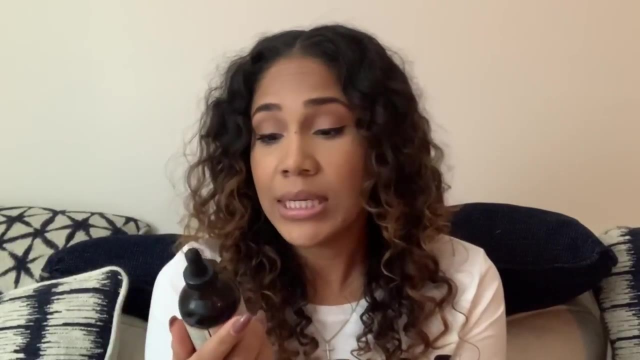 my favorite, um, because a lot of times when kids are hyper it's because they have a lot of yeast in their gut, so probiotic is very important. and the belly balance. there's a barcode over top of it because i don't know why, but the belly balance really is healthy. it's a probiotic blend, um. so 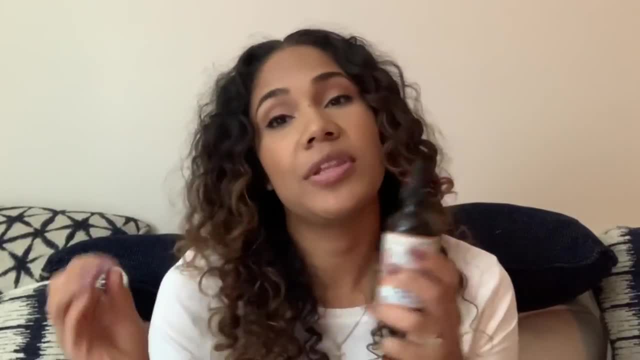 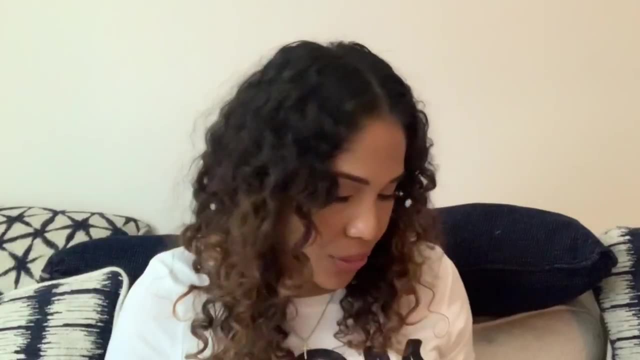 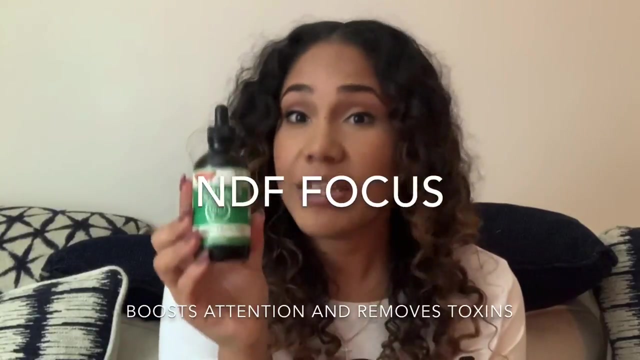 this really helps to keep their gut healthy, which, keeping their gut healthy, helps their whole body. um, so this, we have seen a big change with this as well. and the third one is the mdf focus and it boosts attention and it removes toxins as well. this one has been really 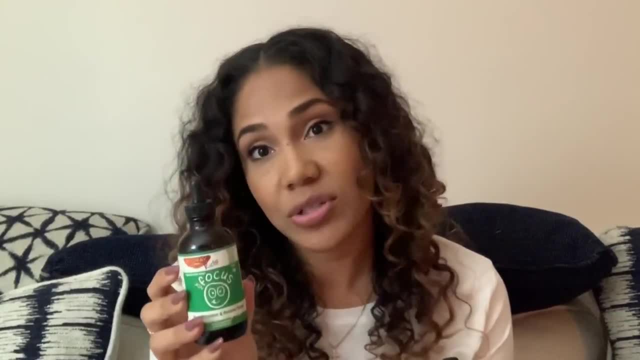 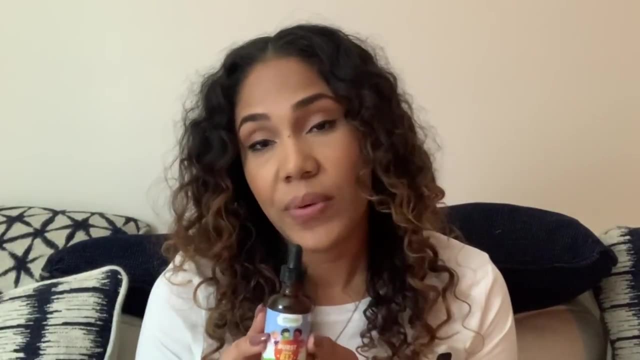 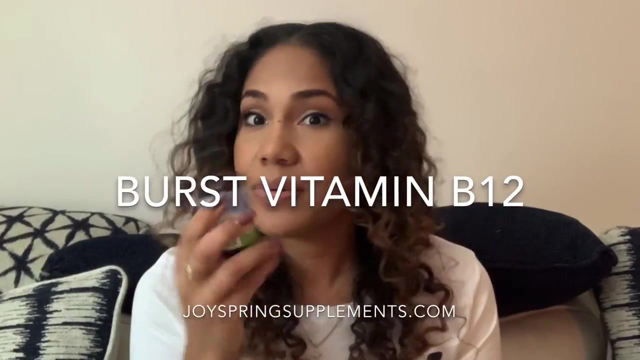 good with getting asking to sit and listen to me when we're doing our exercises and to get him to actually focus. and then one last vitamin that i give him that's not from bio ray is: this is from joy spring, it's the b12. um, my stepfather was talking about earlier one of the main things that he said that was important. 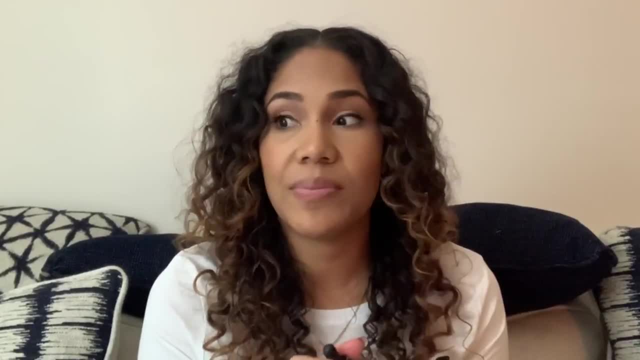 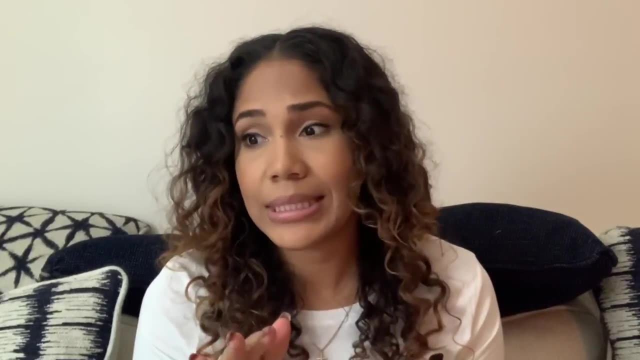 for me to give ashton was b12. he had initially given me this cream that i would rub on his back every single night, and i just figured, because i'm already giving him all of his vitamins, i might as well, instead of adding an additional step at night, to put the cream on his back. why? 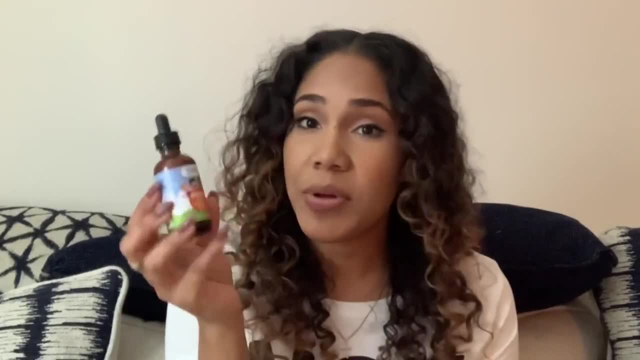 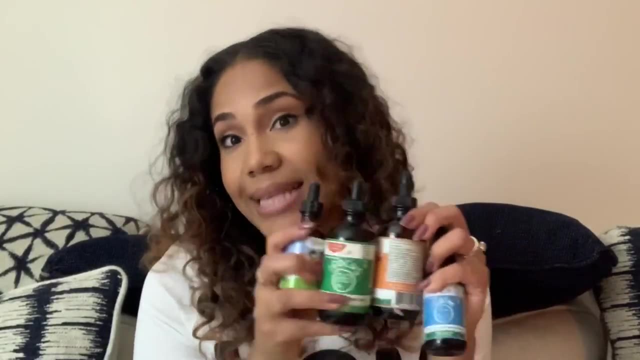 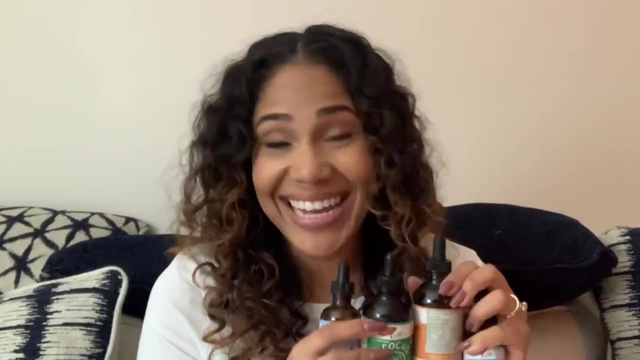 don't i just buy a liquid form of vitamin b12 and put it in there. so those, these four- ashton gets in the morning and he gets at night, in addition to the core four and the adrenal cortex. this is everything that ashton gets. now it seems like a lot. i know it seems like a lot, but after the core, 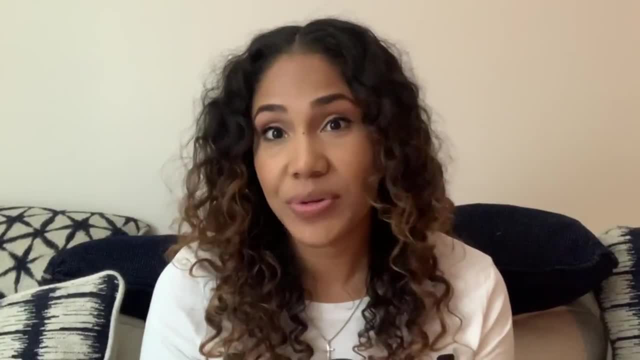 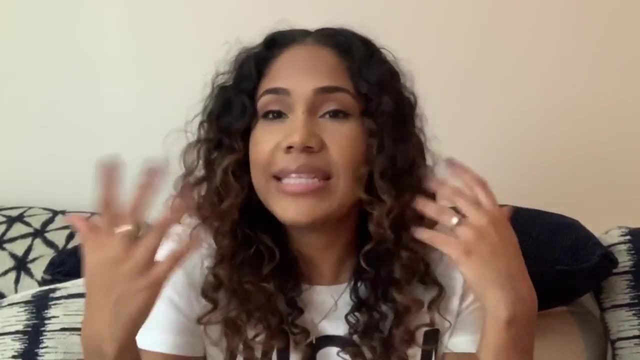 four, just the core four. ashton started answering to his name. he had never answered to his name before. we could call his name, his, call his name. he would look every. he would not even it. it's like he didn't even hear anybody, even talking. he wouldn't make eye contact. 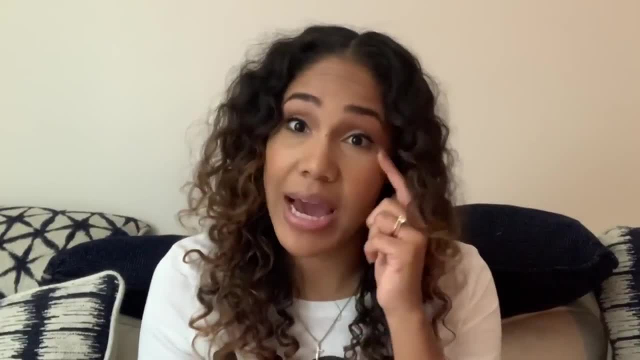 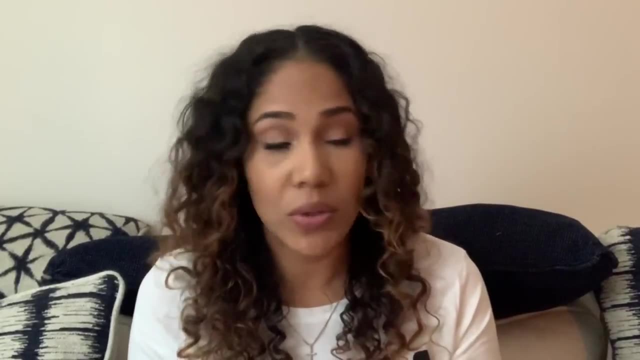 we introduced the core four, he started making eye contact and keeping eye contact. so the core four has changed so much and that was before we even started trying to remove the metal once we did biore- i'm not gonna lie- in the beginning i was like, okay, we don't see any. 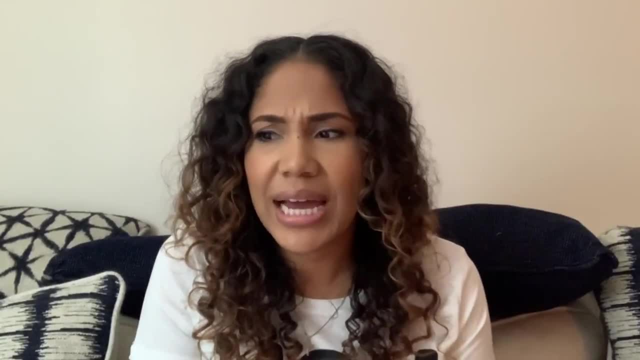 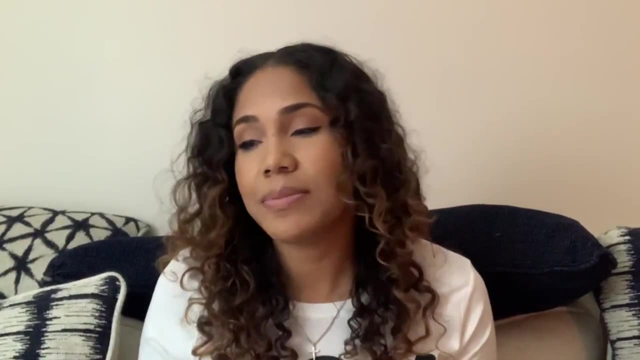 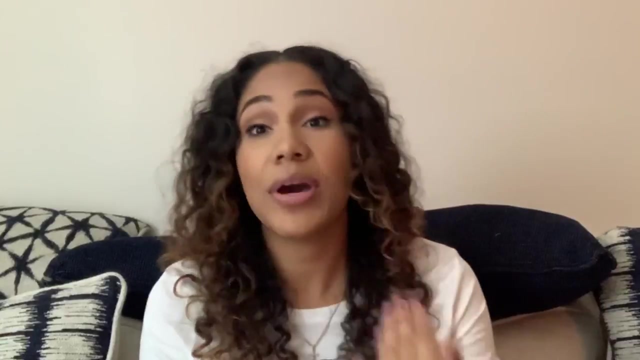 anything. um, it had been like four weeks, almost five weeks, and i'm like yo, we are giving him these things religiously. and i remember i looked up some reviews and they were like just wait, by week five he was a totally different kid. he would come up to me to play, he would come up to me to read him books. 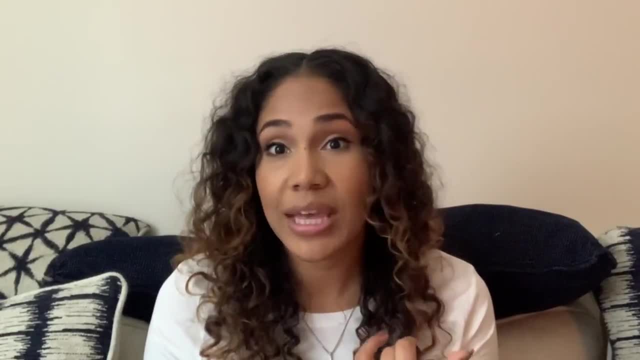 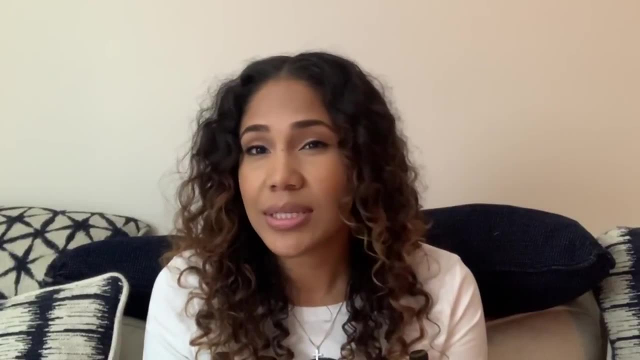 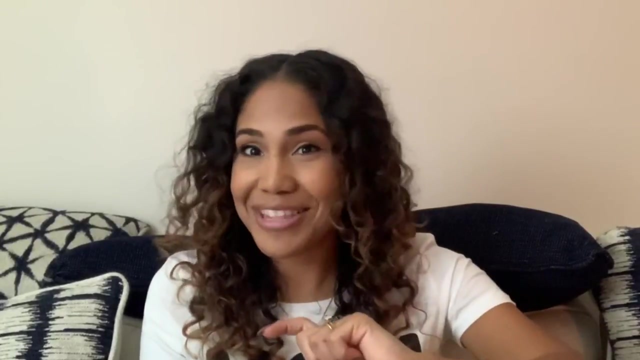 he would sit and listen. he- i go over animal sounds with him and he's mimicking them. now, mind you, ashton says the words uh, but he mostly focuses on the vowel and doesn't really complete the consonant. so that is something that we're working on, but this is coming from a kid. 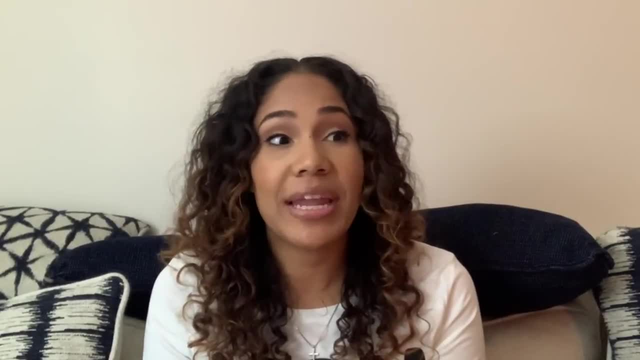 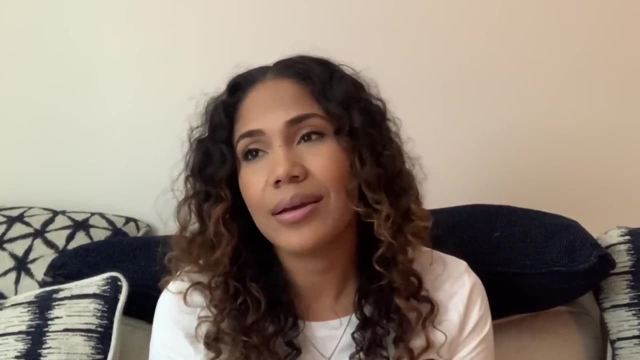 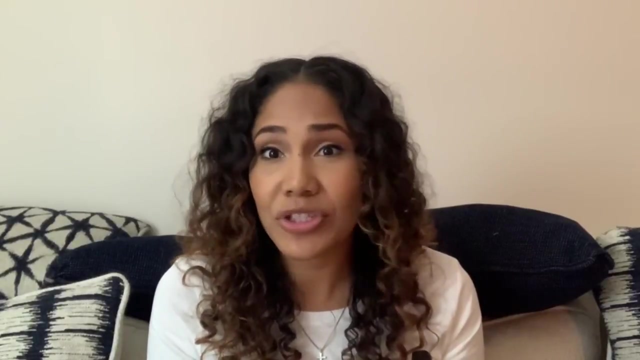 who never will repeat anything. this is coming from a kid who would never say hi or bye. now he's way time by. um. he says: i will you, or it's like i love you like that, but i'll take it. it's like i love you, i'll take it. um. he says cheese to take pictures when i'm brushing his teeth instead of me being. 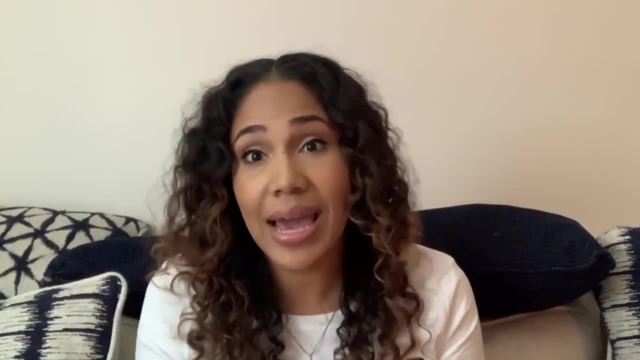 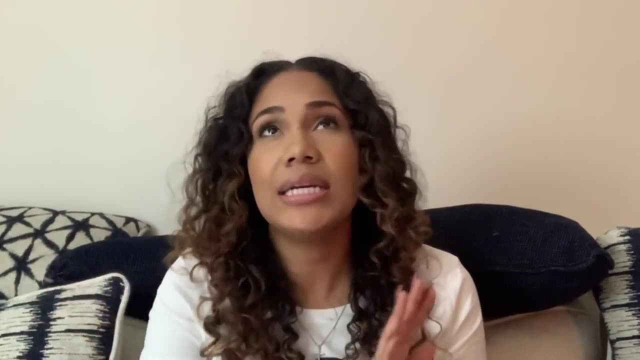 on top of him trying to hold his mouth open to brush his teeth. if i say, say ah, he says ah, he lets me get to his teeth. it's still a struggle brushing his this man's teeth okay, but it's a vast improvement. so i would definitely recommend biore kids. 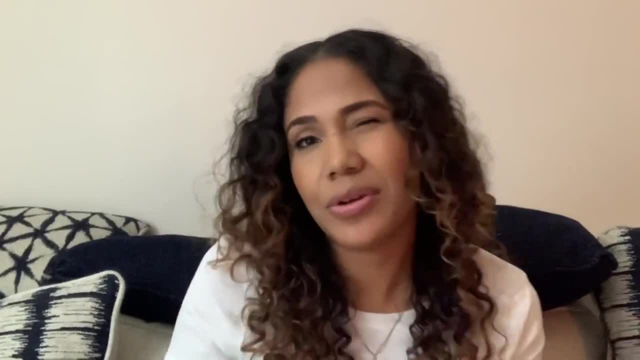 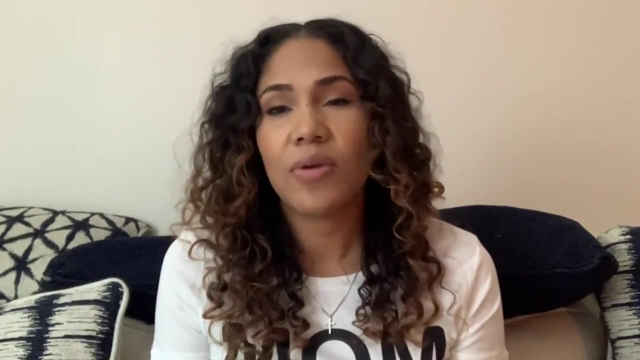 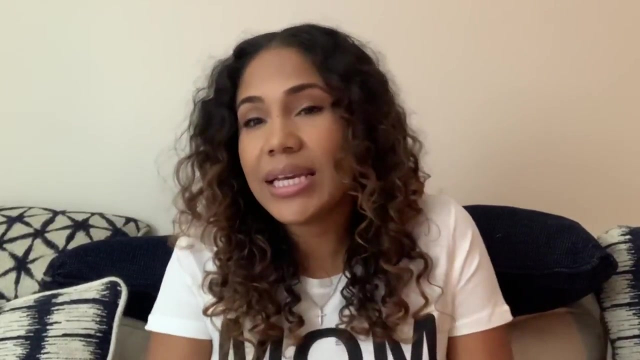 think it's safe, um, starting at 12 months, but you have to read on things. i i am very impressed, i am very grateful because they really have helped so much. it does seem like a lot in the beginning, um it, it can be a little tedious, but once you get into the groove, i send ashton's vitamins to school. 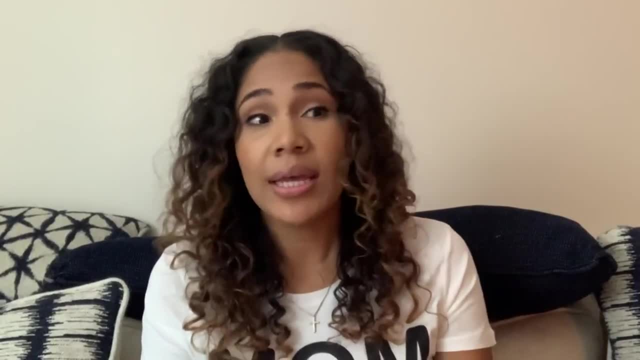 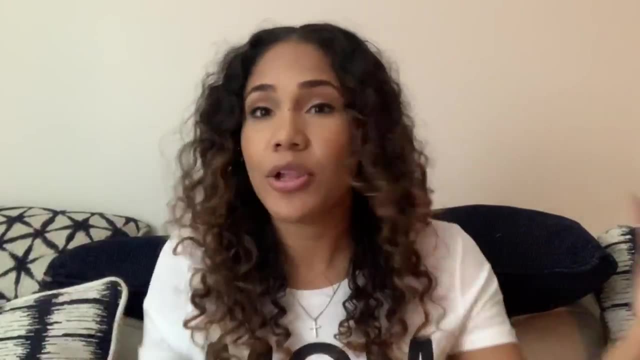 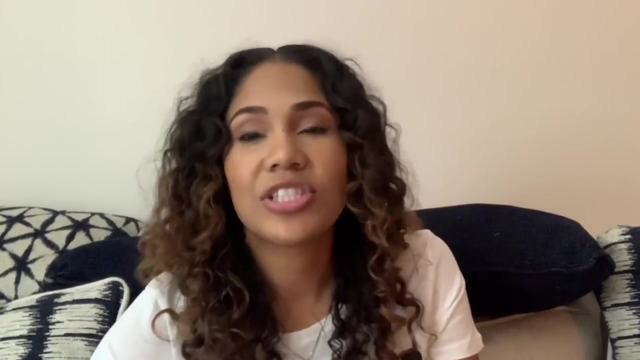 for during the day and they give it to them in his juice and you know it. just, the system just works and he just it's like he's waking up and he's just alert and he's here and i'm loving it and i'm so grateful and i'm so happy. you guys should definitely look into it again. start with this book. 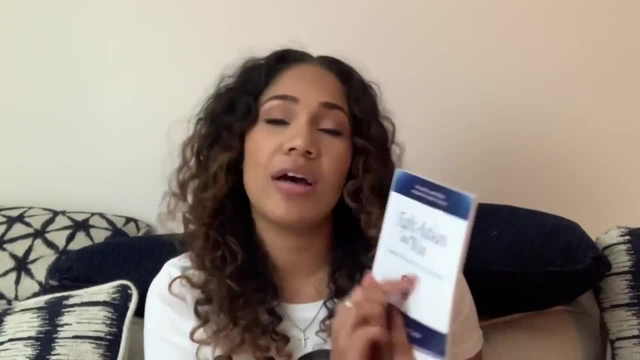 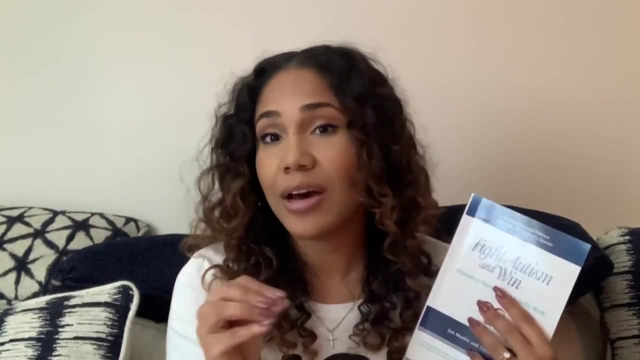 even if your kid doesn't have autism. start with this book: fight autism and win it. it is really incredible, and it's it. it's chock full of information that can help your child, regardless on if they're on the spectrum or if they just have a delay. it's, it is really, really incredible. so.